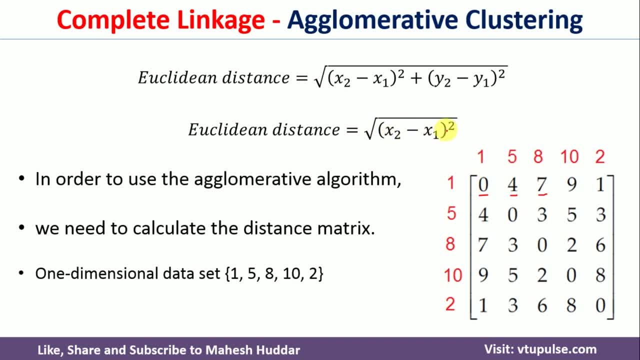 square root of 8 minus 1 bracket square square root will get cancelled. we will be left with 7 here. Similarly, we can calculate 9, 1, and so on. So all these particular distances are calculated using this particular formula here. Now, once you. 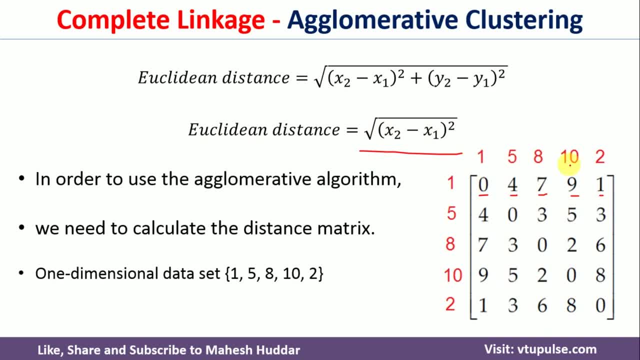 calculate these particular distances. actually I should write the column number and row numbers over here, Just for understanding purpose. I have written this particular actual data over here, So I will replace this particular actual data with the column numbers here. 1, 2,, 3,, 4, 5 are. 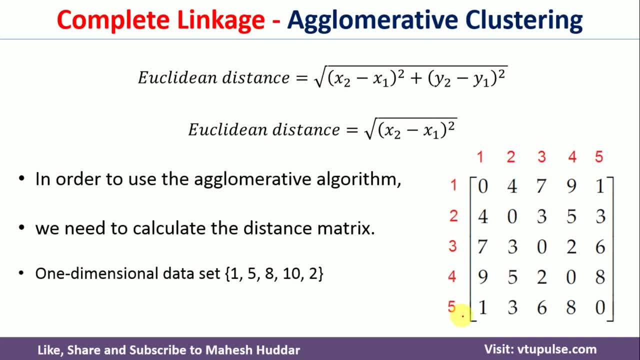 the column numbers, and 1,, 2,, 3,, 4, 5 are the row numbers. These are the distances, what we have calculated right now. Now, coming back to the next part of our discussion, what we do over here is whenever we want to apply algorithmic hierarchical clustering algorithm. given this, 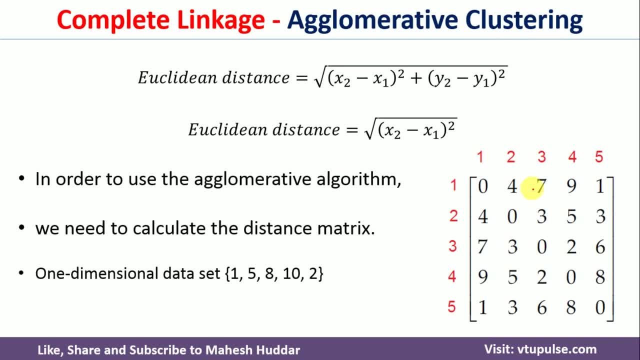 particular distances. we will try to identify the minimum distance And if you look at this particular matrix, this is the minimum distance. what we can notice that is between 1, 5, or you can say that 5, 1, that is the minimum distance. Now what we do over here is because the 1, 5 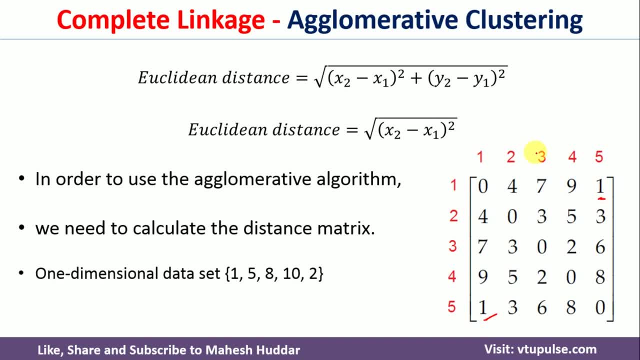 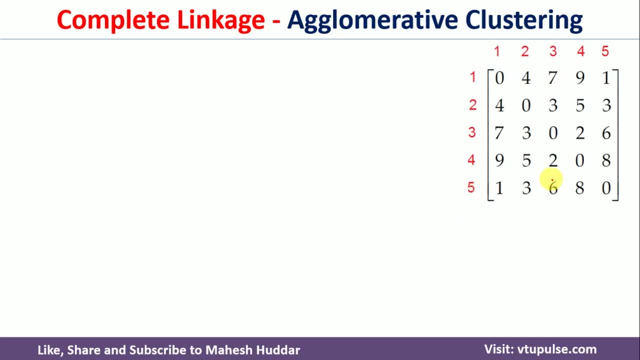 is having the minimum distance. we will club this particular 1, 5 into one cluster, and the distance till here is 1 in this particular case. Now, once you group that particular thing, the next question comes in front of us is: we have to. 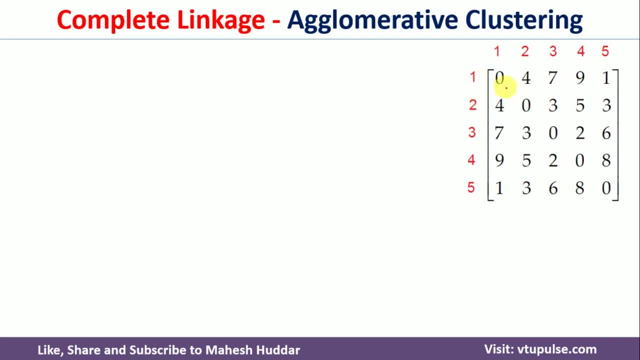 calculate the distance from 1, 5 to 2, 1, 5 to 3, 1, 5 to 4, because we don't know the distance from 1, 5 to 2, 1, 5 to 3, 1, 5 to 4 here. So what we do over here is here we will apply the complete. 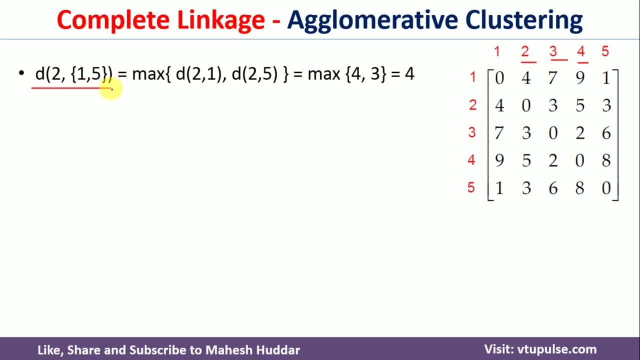 linkage formula, that is, we will try to find out the distance between 2, 1, 1, 5, or you can say that 1, 5, 2. So both are reflexive in one another. So that's the reason we will calculate one distance over. 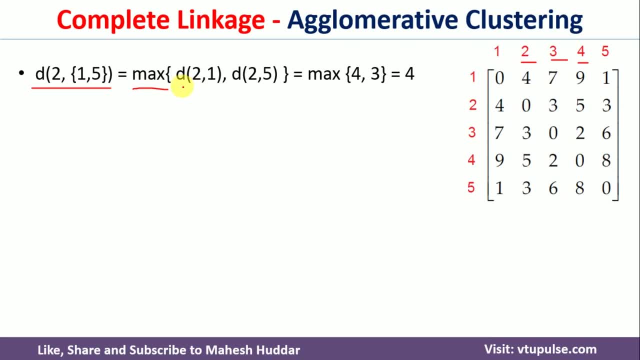 here that is always equal to maximum of d 2, 1, d 2, 5, that is, 2, 1 and 2, 5.. What is distance between 2, 1?? The distance between 2, 1 is equal to 4.. Distance between 2, 5 is equal to 3.. The 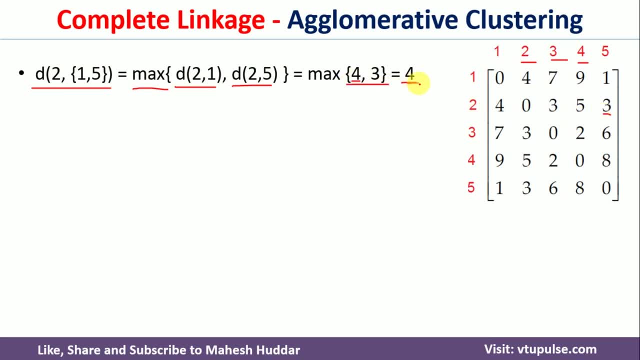 maximum between these two is equal to 4 over here. That is nothing. but distance between 2, 1, 5, 2 is equal to 4.. Similarly, the distance between 1, 5, 2 is also equal to 4 over here. Similarly. 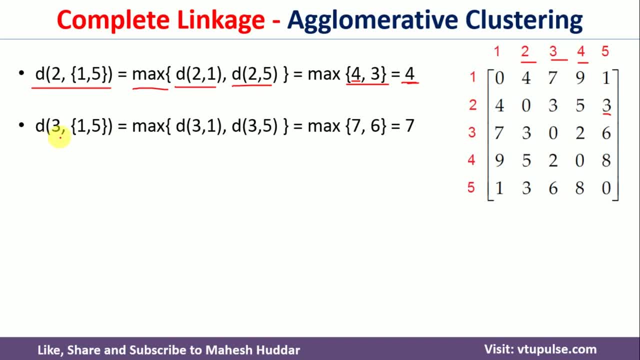 we will calculate the distance from 3 to 1, 5, 1, 5 to 3 over. here Again the same formula we will apply, That's a maximum of d of 3, 1.. 3, 1 is how much That is 7.. I have written it here. 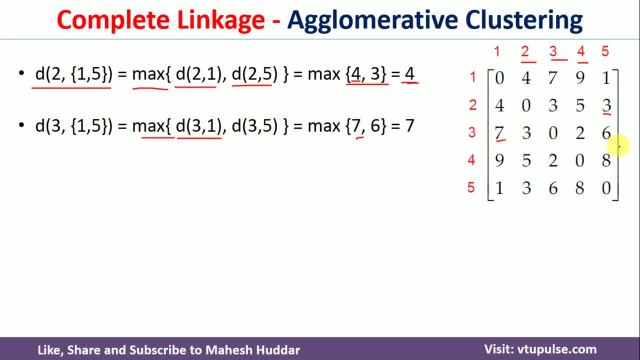 D of 3, 5.. 3, 5 is 6.. That is 6 is written here, and the maximum between these two is 7. over here, Distance from this 4 to 1, 5, that is equal to 9 in this case. Now, what we do over here is we will. 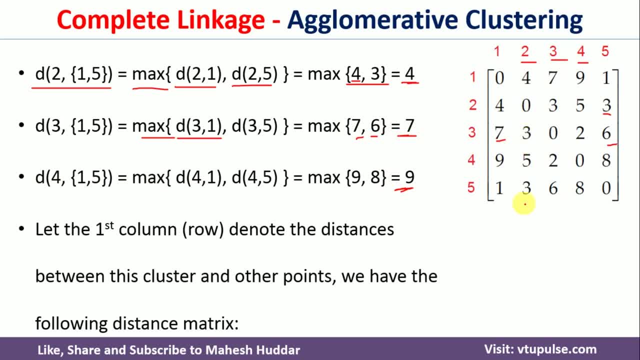 try to write the modified matrix over here. That will look something like this one: 1, 5 over here. 1, 5 over here. that is nothing but one cluster. we have created Now from 1, 5 to 2,. what is the? 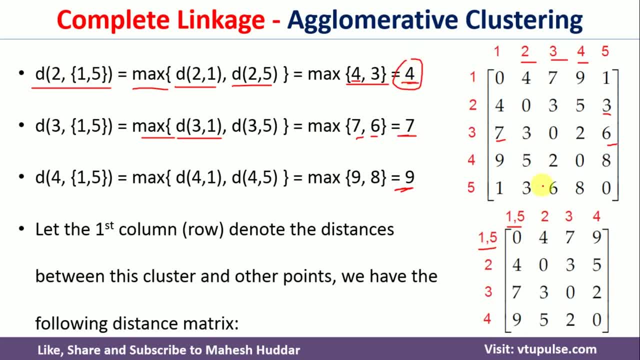 distance we have calculated. That is nothing but 4 here. So that is what I have written here: 1,, 5 to 3, what is the distance we have calculated? 7 here. I have written the same thing here. 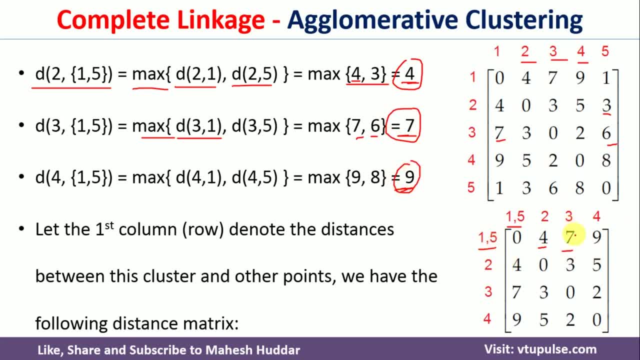 1, 5 to 4,. what is the distance we have? That is 9.. The same thing will come over here in this particular column, That is 2 to 1, 5, 3 to 1, 5, 4 to 1, 5 here, And these values are already available in that particular matrix. We 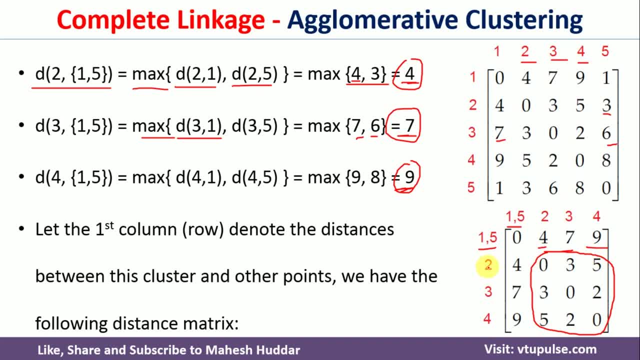 have not modified these things. For example, 2 to 2, what is the value we have here? 0.. 2 to 3, what is the value we have here? 3.. And 2 to 5, what is the value we have? 2 to 4, actually. 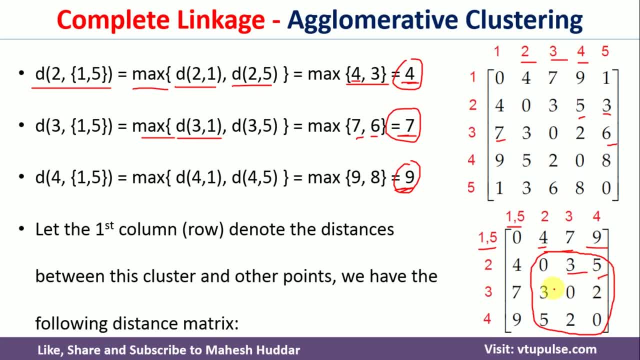 the value is equivalent to 5 here, So that is not modified. So we don't worry about these things. Now, once you create this particular modified matrix, again we will try to identify the minimum distance in this particular case. If you look at this: 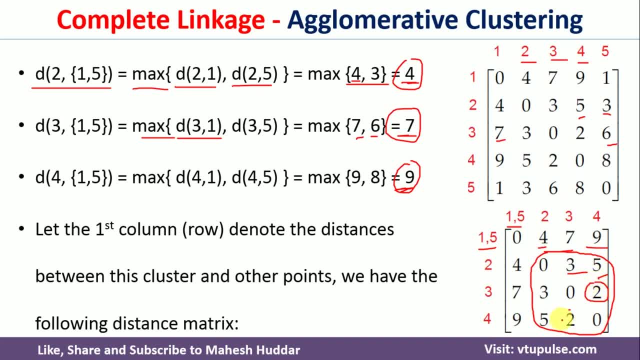 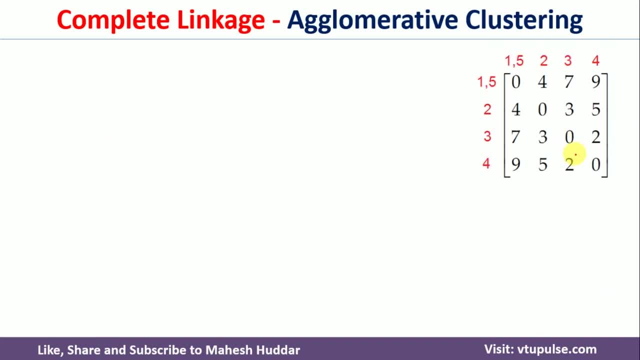 particular matrix carefully. this particular distance, that is 2, is the minimum distance in this case. that is between 3 and 4 over here. So because we have that particular minimum distance over here, what we will try to do is we will try to club this particular 3, 4 into one cluster. 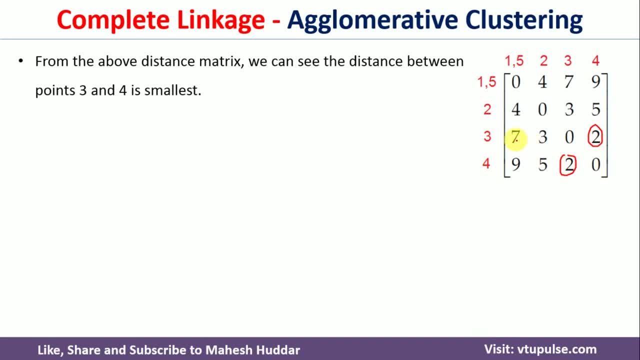 Now, once you club that particular 3, 4 into one cluster, what will be left with us is 1,, 5,, 2 and this 1, that is 3, 4.. So this is 1 cluster. here Again, we need to identify what is the distance between 1, 5 to 3,. 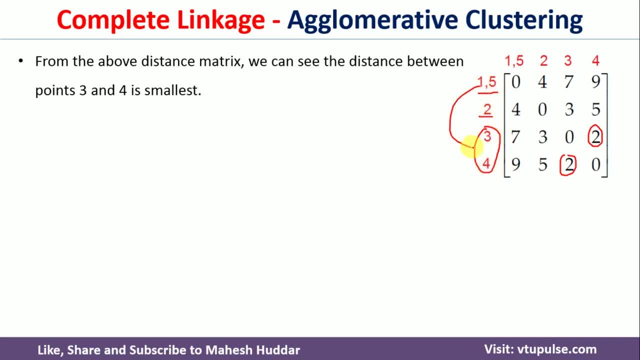 4 as well as 2 to what is that called as 3, 4.. Because we already know what is the distance between 1, 5 to 2, there is no need to calculate, Because we have created a new cluster here. 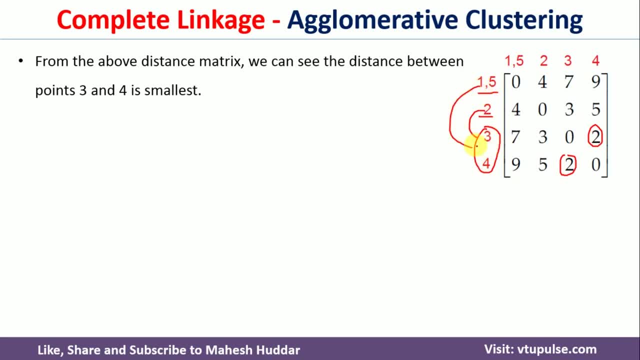 we need to calculate the distance between 1, 5 to 3, 4 and 2, 3, 4 over here. So that is done. something like this: The distance between 1, 5, 3, 4 is equivalent to: 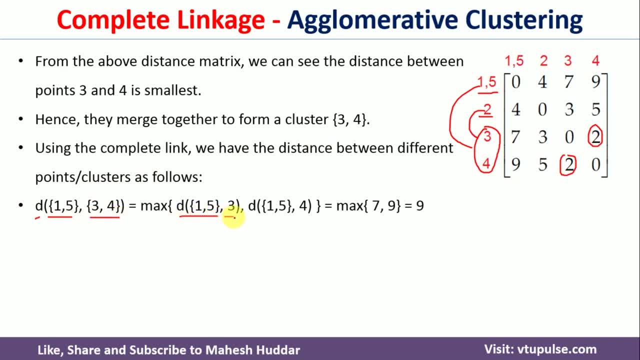 the distance between 1, 5, 3, distance between 1, 5, 4 over here: 1, 5, 3 is equivalent to what We have 7 here. that is what I have written here. 1, 5, 4, that is 9, I have written here. 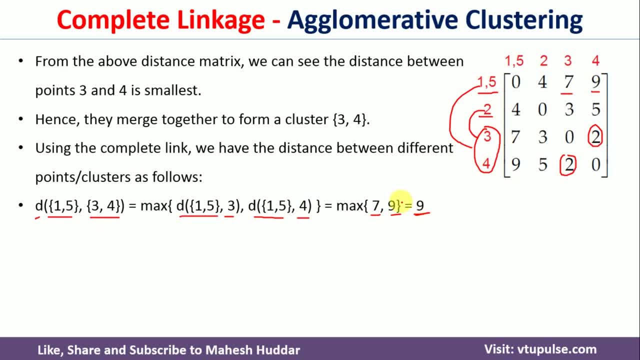 and the maximum between these two is 9 in this case. Similarly, 2, 3, 4,, that is, 2 to 3, 4,. we need to identify distance between 2 to 3 and 2 to 4,. we need to identify the distance between. 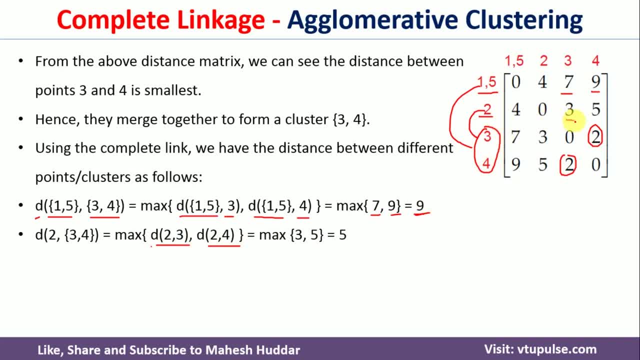 2 to 3.. If you notice here 2 to 3 is 3 and 2 to 4. is equivalent to 5. between these two, 5 is the maximum over here. now we need to write that particular modified matrix over here so we will get 1 comma 5, 2 and 3 comma 4 over here. 1 comma. 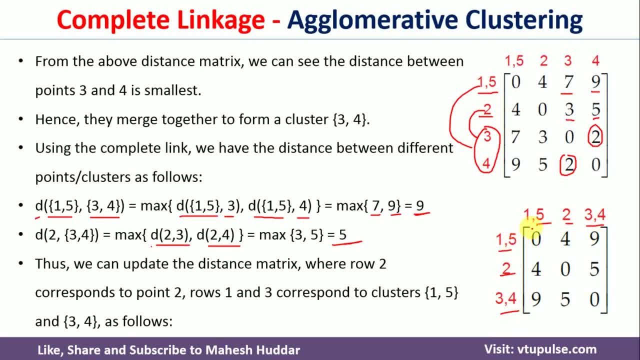 5, 2, 3 comma 4 over here. 1 comma 5 to 1 comma 5. we know this one: 0, 1 comma 5 to 2, which is already known to us, that is 4. i have written it as it is: 1 comma 5 to 3 comma 4. we have calculated it here. 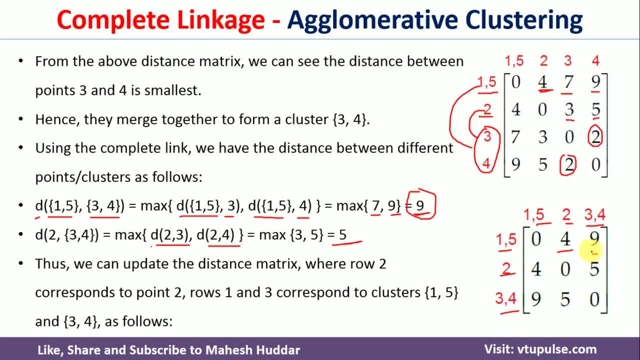 that is equivalent to 9. i have written it here now. 2 to 1 comma. 5 is already known to us. that is 4. i have written it as it is. 2 to 2 is equivalent to 0. 2 to 5 is equivalent to, not 2 to. 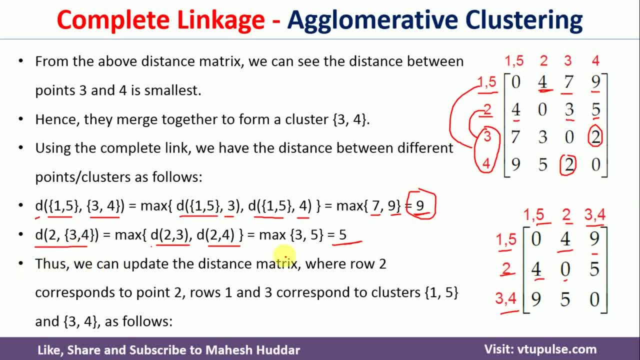 5. 2 to 3 comma 4. we have calculated it. that is nothing but 5. we have already written it here. now: 3 comma 4 to 1 comma 5. that is reflexive in nature. so the 1 comma 5 to 3 comma 4 and 3 comma. 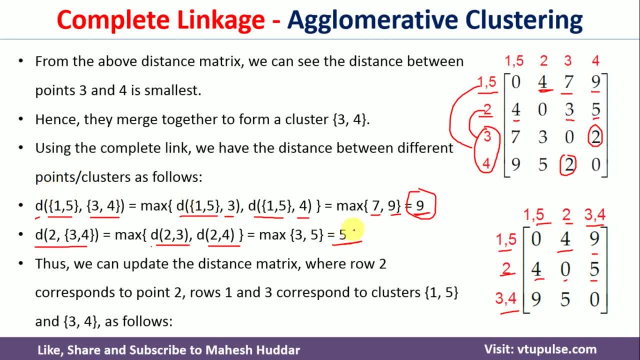 4 to 1 comma 5. both are one another same, so that is nothing but 9 here. i have written it here: 3 comma 4 to 2, that we have already calculated. and i have written it here: 3 comma 4 to 3 comma. 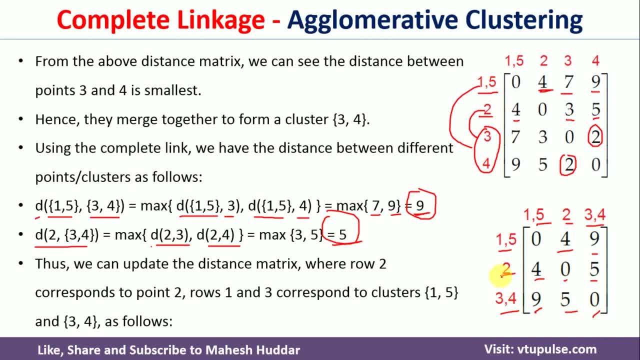 4 is equivalent to 0: 0 here. so now we have written this particular modified matrix, now we need to check which is the minimum distance from this particular thing and if you look at this particular matrix again carefully, the 4 is the minimum distance. now what we need to do is we need to club this particular 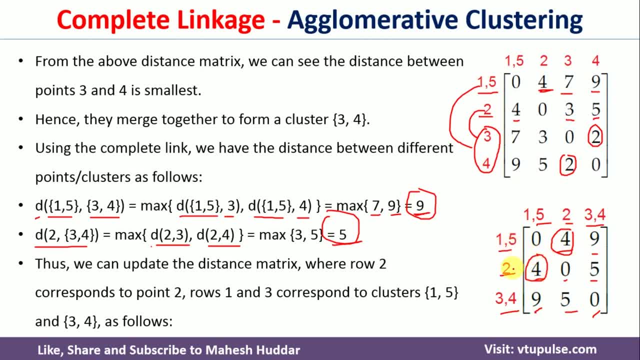 1 comma 5 comma 2 over here. this will be one cluster and another cluster will be 3 comma 4 here. now, once you combine this particular thing, we need to identify the distance from 1 comma 5 comma 2 to 3 comma 4 here. so if you club this particular thing and if you want to identify the 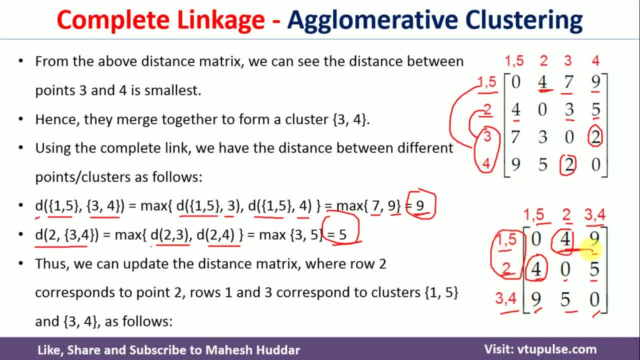 distance between these two things. we need to check what is the maximum between these two. that is what we have done over here. so what is the maximum between 4 comma 9? 9 is the maximum over here. so that's the reason. the distance from 1 comma, 5 comma 2 to 3 comma 4 is equivalent to 9 in this. 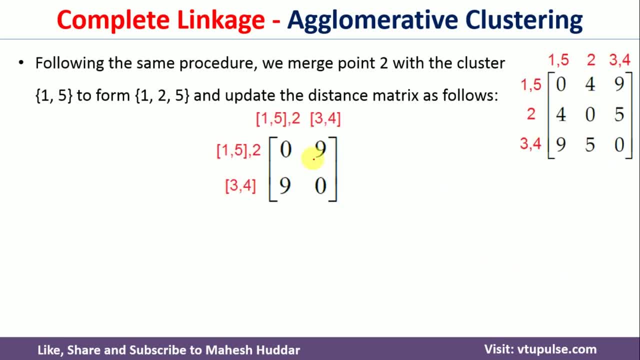 case. so that is what i have written in this particular case. so this is the first cluster and second cluster, from this particular thing to this one. if you notice here, between these two, which is the maximum, 9 is the maximum. so that is what i will write here. 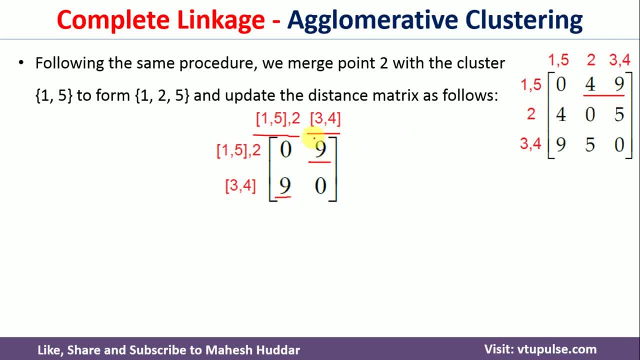 and the reflective value is written over here. so this is what actually the next matrix, what we got and what is the distance. right now the distance is 4 here. the first time, when we clubbed 1 comma 5, the distance was 1. when we clubbed 3 comma 4, the distance was 2. when we clubbed 1 comma 5, comma 2. 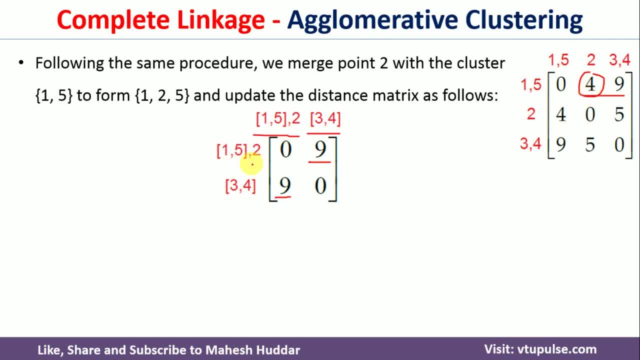 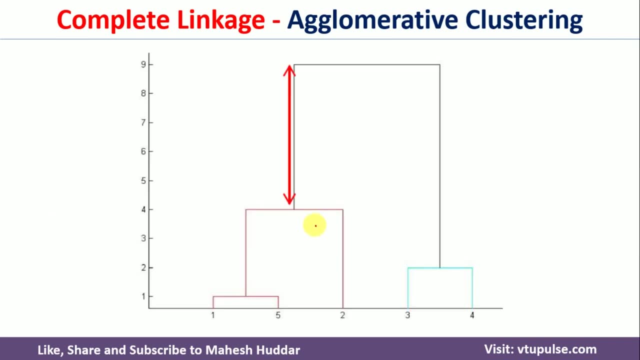 the distance is 4 here. now, when you combine these two things, that is 1 comma 5 comma 2, that's the first cluster, and 3 comma 4, that's the second cluster- the distance will become 9 in this particular case. now, once you merge all this particular thing, the dendrogram looks something like this: that is when 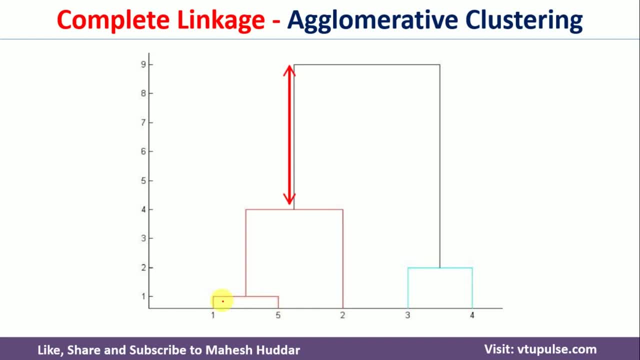 i have combined this particular 1 comma 5, the distance was 1, so that's the reason we have to keep this particular thing up to here. and when i have combined 3 comma 4, the distance was 2, so i have to keep it up to here. and when i have combined 1 comma 5 and 2, the distance was 4, so that is the.